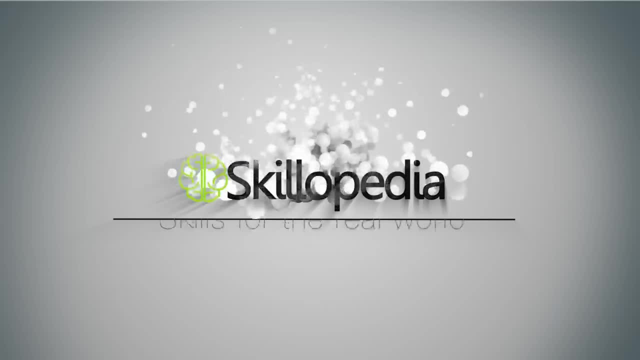 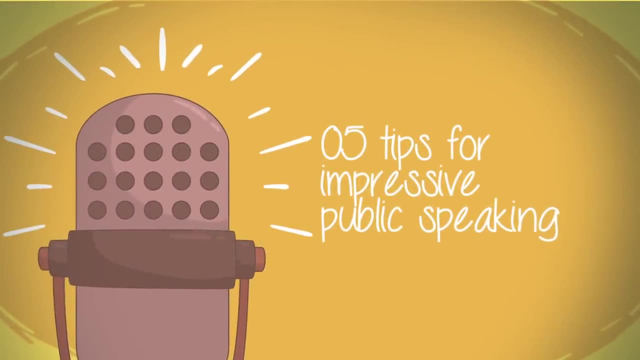 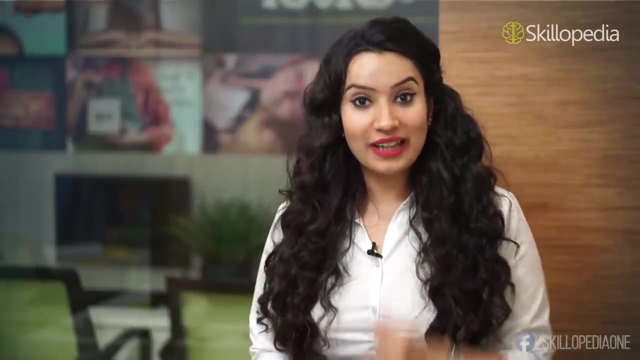 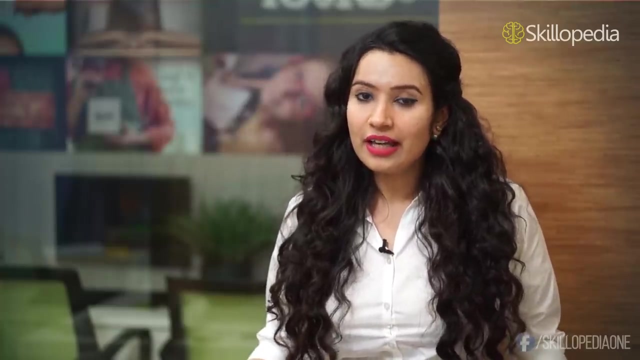 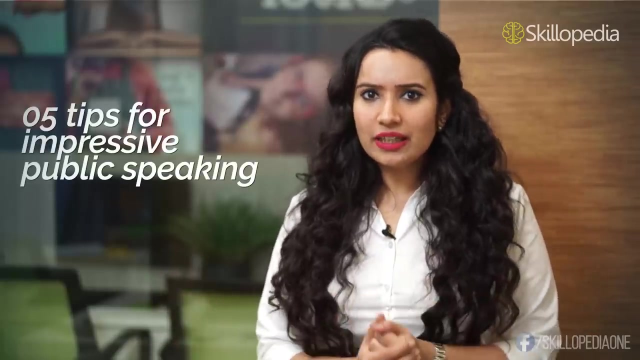 Speaking in public is a challenge, and a challenge I believe must be accepted. What do you think? We all have that moment on the stage when we go blank. Have you ever freezed on the stage? Well, I have seriously freezed on the stage once at my school, Speaking in front. 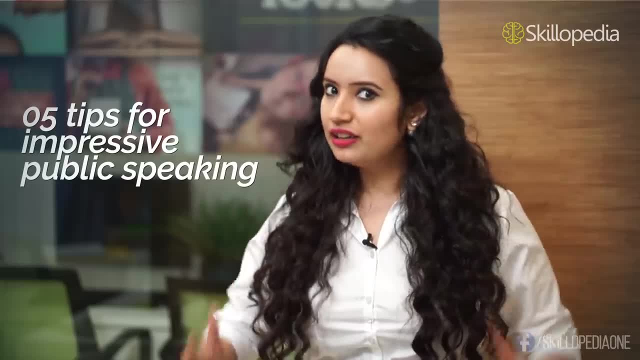 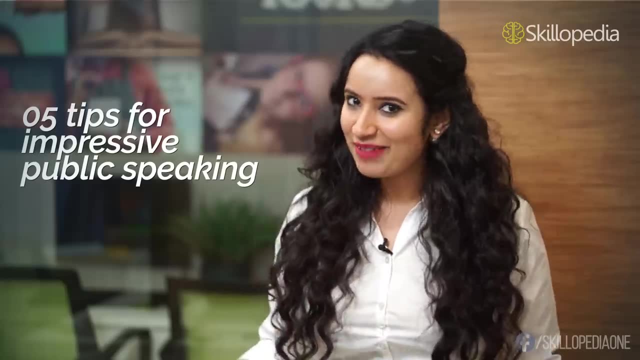 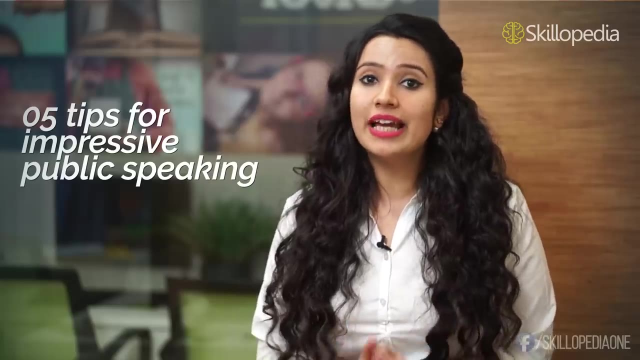 of the crowd means having to go through sleepless nights, nervousness, deadlines and many rounds to the toilet when you're just about to start, Am I right? Okay, guys, my name is Michelle and today I'm going to share with you some valuable suggestions that will help you speak. 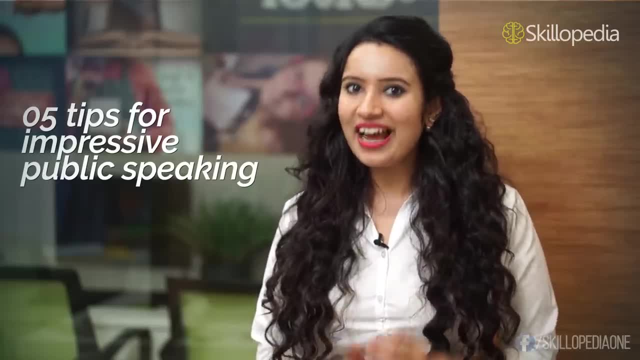 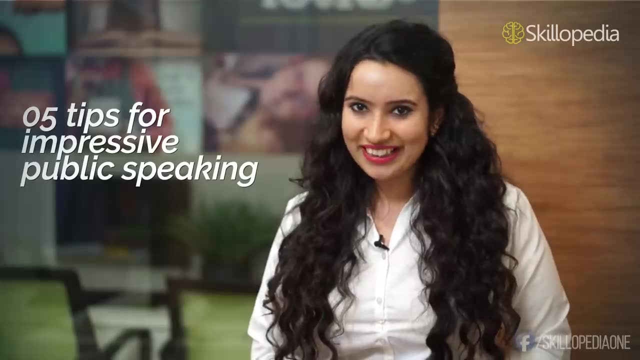 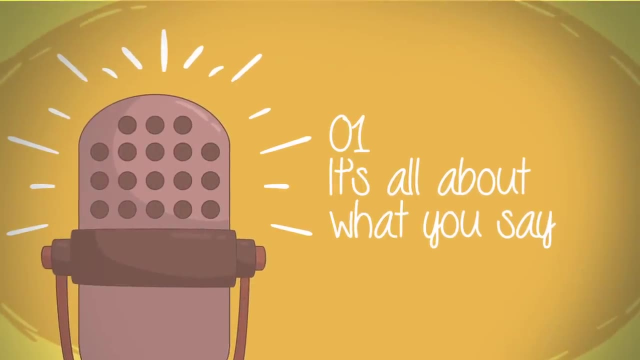 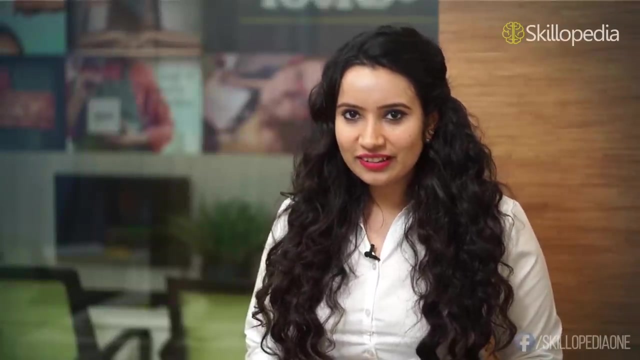 better publicly. So stay tuned to this session, as I share some tips to help you understand the mistakes that you've been committing all this while, while speaking publicly, You're watching Skillopedia, the place to learn skills for the real world. There is an age old saying: a good speech is like a pencil: It has to have a point. 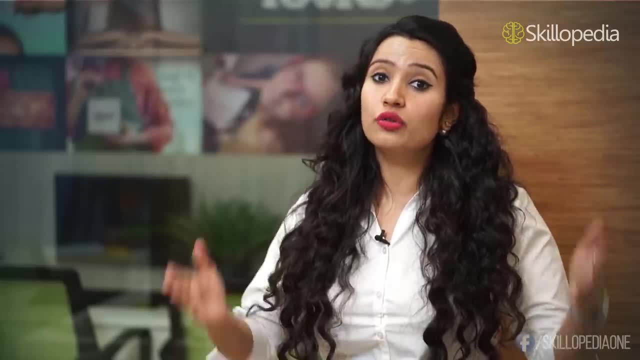 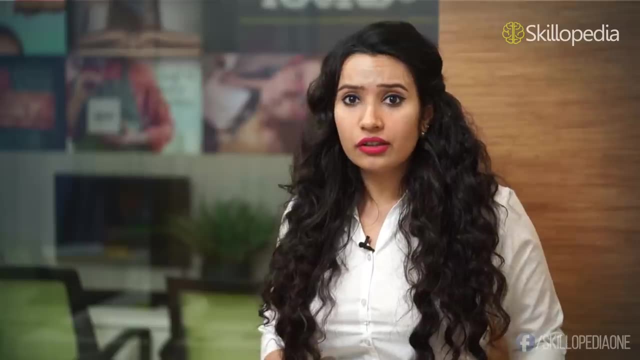 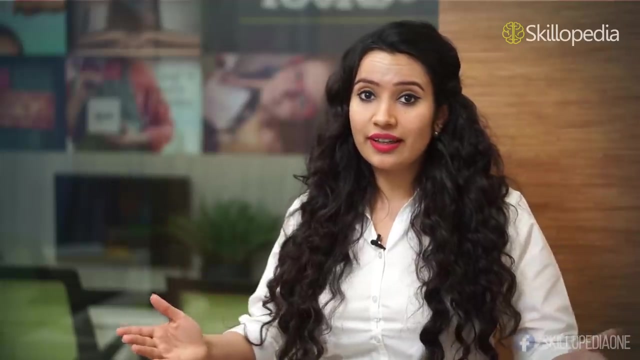 For this very reason, you might sit the entire week to frame the right points by adding some big words and some very good vocabulary to make it look good. You might also make enough PowerPoint presentations with pictures, graphics and figures, But you're losing on something. 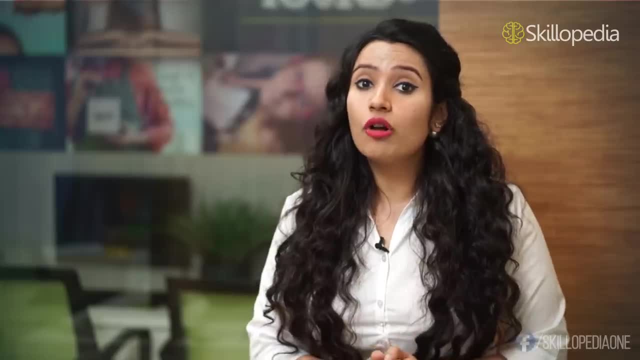 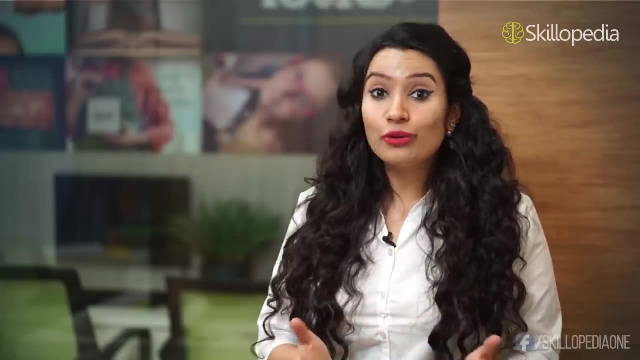 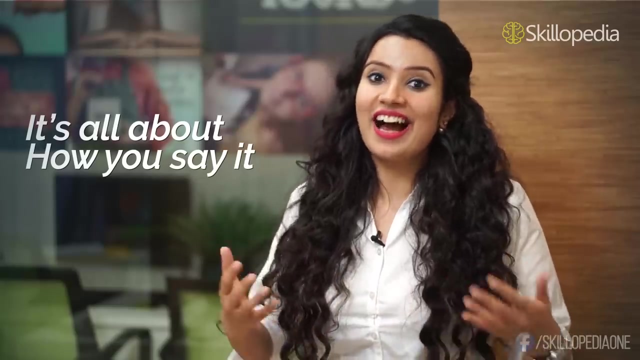 here, The majority of your time would be spent on preparing the content for the event, as in what you're going to speak. But what we miss out is how to speak. We spend a lot of time thinking what to say, But not enough time thinking how to say. So let me give you a heads up. I mean, let me 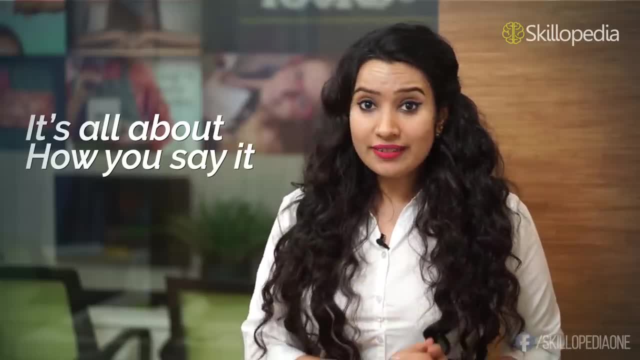 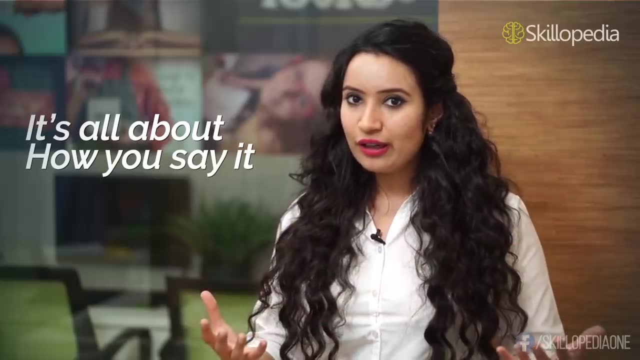 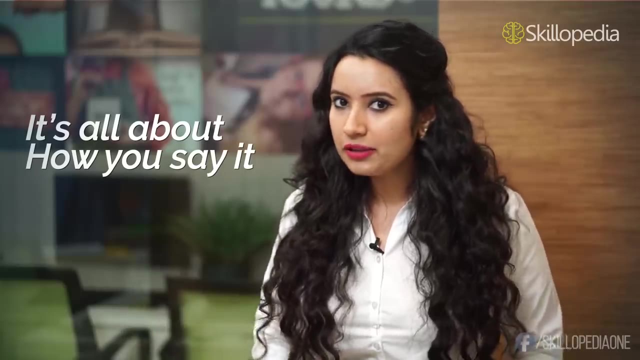 tell you how the figures are. Researchers say that lasting impression is more directly tied to our voice and body language. So, to my shock, content and words play only 7% of the role in communicating, And I was absolutely surprised to find out. Then what does the other? 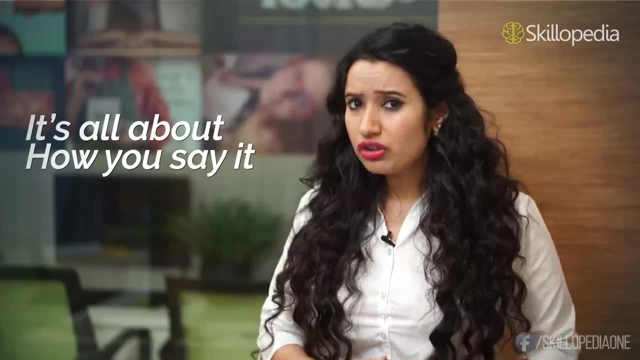 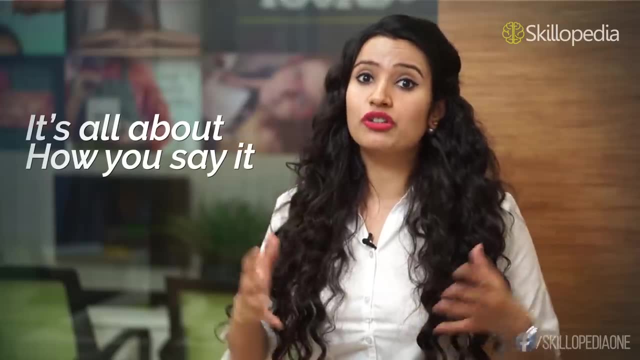 93% depend on. Well, the other 93% depends on how your body language is. How much of 10% depend on? If it's not about what you're saying, then voice takes 38% and body language 55% of what you're speaking. Isn't that a shocking statistic to you? A person's ability? 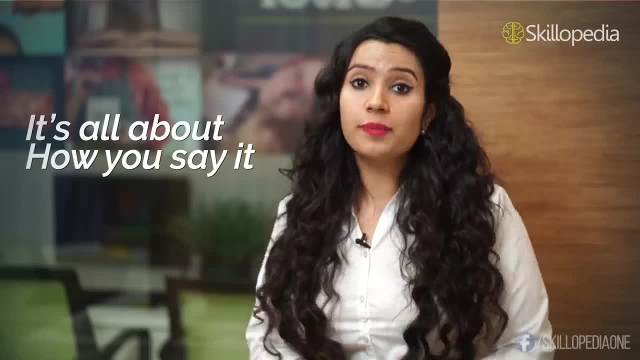 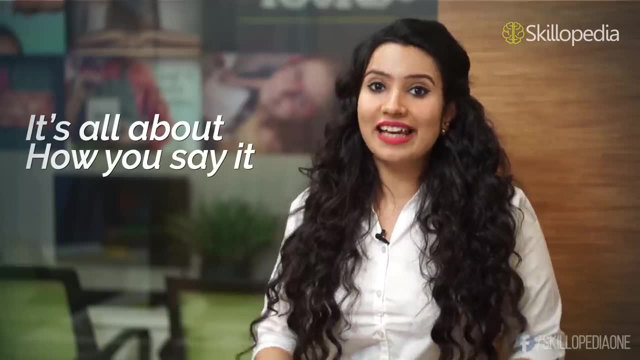 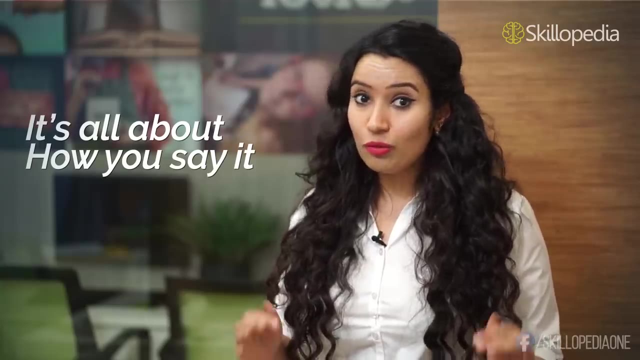 to speak and communicate to an audience largely depends on the body language rather than on the content, rather than on what you're speaking. So body language is like a text you send to a friend. If you're polite and funny, the vibes are good, But if you put in sarcasm, 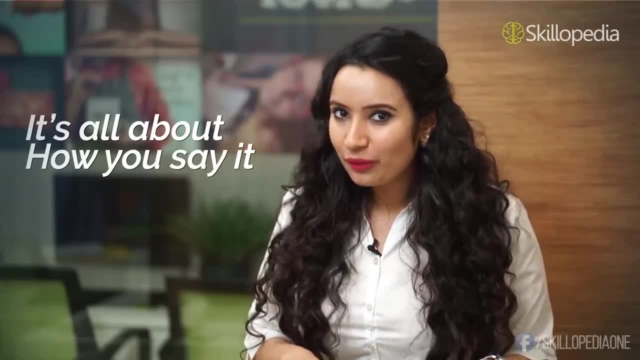 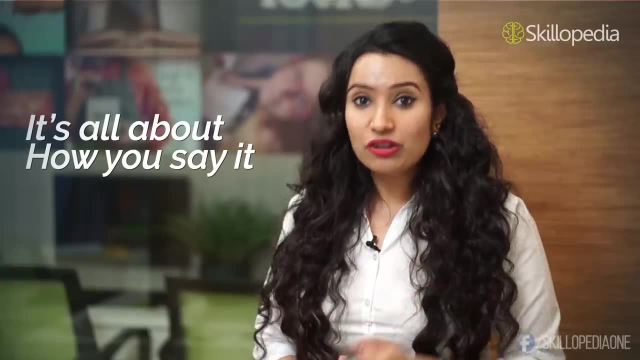 you mess up the good conversation. So if your body language is not nice, you mess up your entire relationship with the audience during the public speech. So make sure you don't hurt the sentiments of the people who are listening to you. Rather, you focus on a positive. 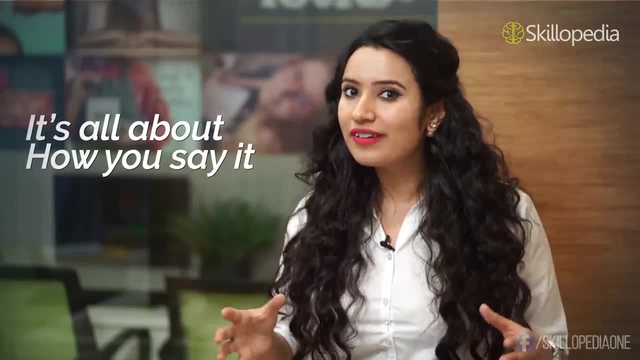 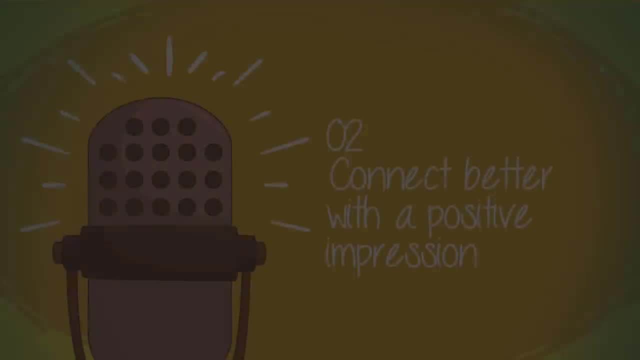 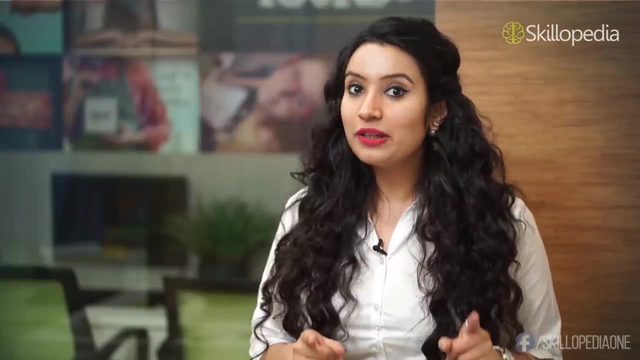 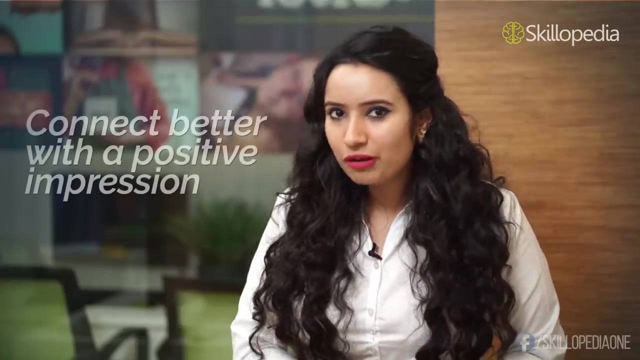 and happy way to deliver your speech, which is best reflected in your body language and your voice. So concentrate on how to say more than what to say. First and foremost, it's important that we not only make a lasting impression, but that we make a positive one. Yes, let me tell you about my professor back in college. He was 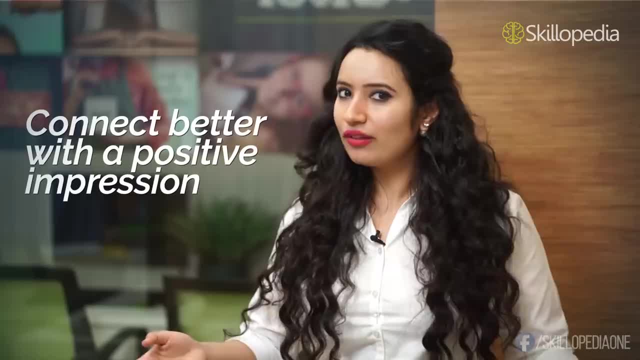 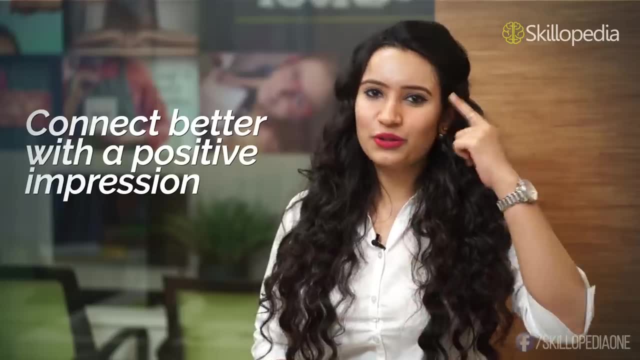 a kind of weird guy. He would take long pauses while speaking like this, but whenever he spoke he would say something like I could not remember what he said. I was just kind of lost for words. I could not remember what he said because I could not remember what. 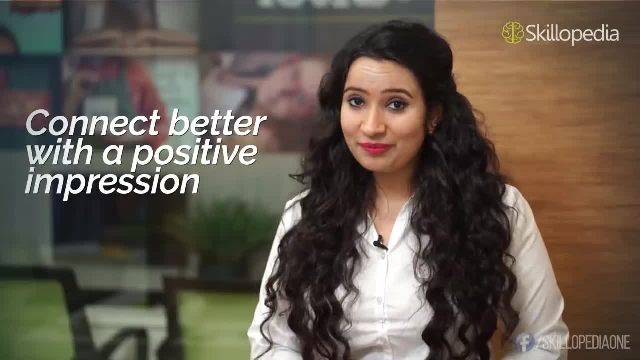 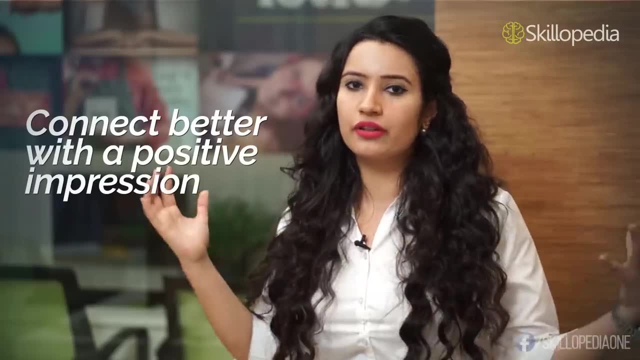 he said, And he just had a great sense of humor on top of that, And that is what attracted most of the students from my class. We all came from different parts of India and different parts of the world, But when we heard him, we were all laughing on the same joke and 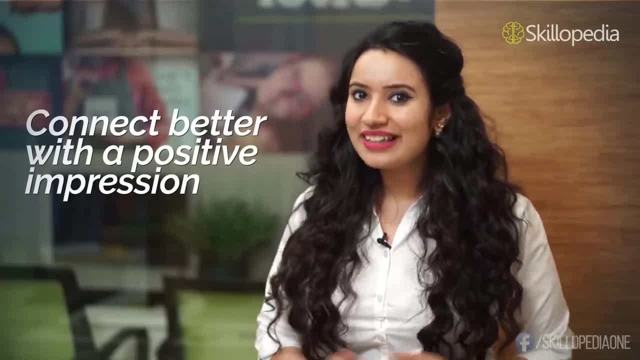 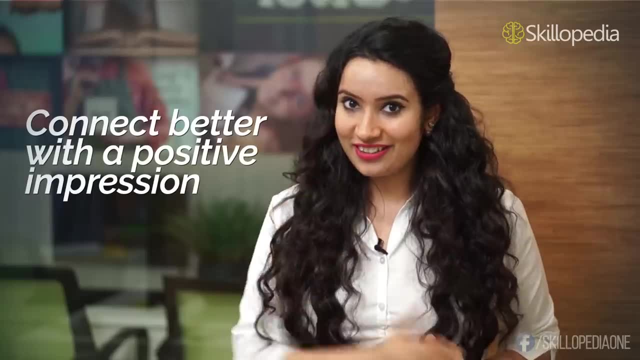 listening to him very carefully. But apart from humor, it's important to look at your audience. That's what he did When he took those pauses. He used to look at us. That's look at us. So don't keep your eyes fixed on a spot, rather watch across the entire hall. 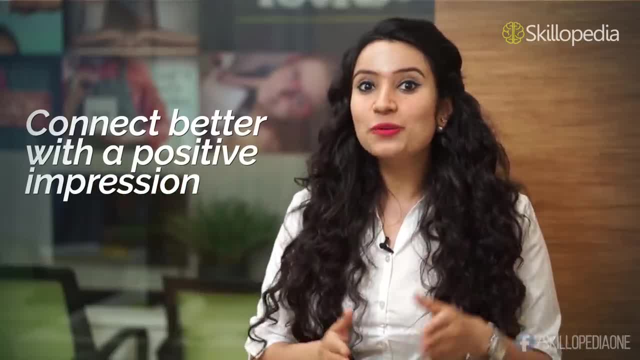 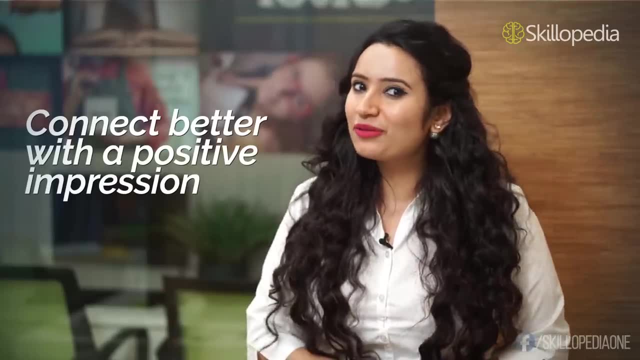 making meaningful eye contact with your audience. This will help you connect better to them, and there is no better way of explaining a point than using examples from daily life. Like I'm telling you about my professor, you could also tell about one of your experiences. 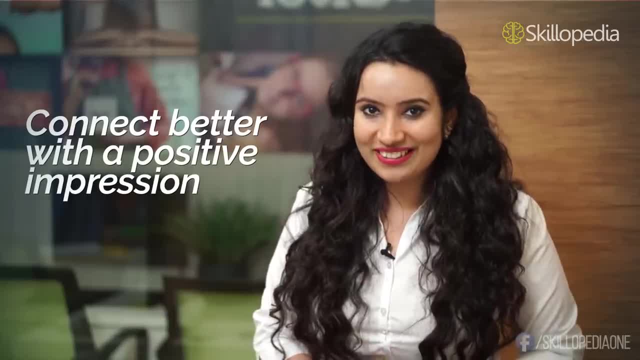 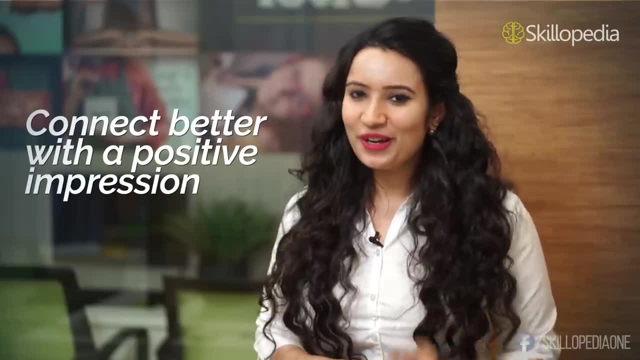 from your school or your college days, or maybe even from your workplace, because examples help to relate to the topic much better than anything else. Trust me, I used them too. So you must add examples. have a nice body language and look at your audience and you're. 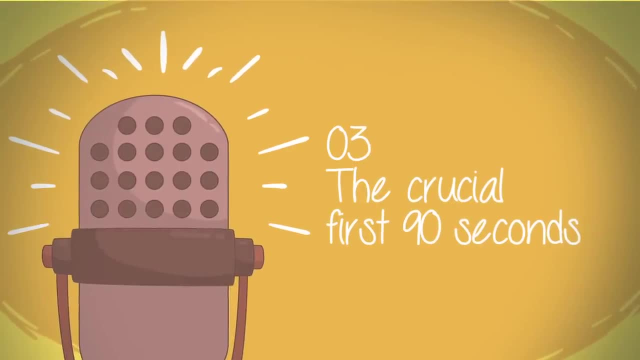 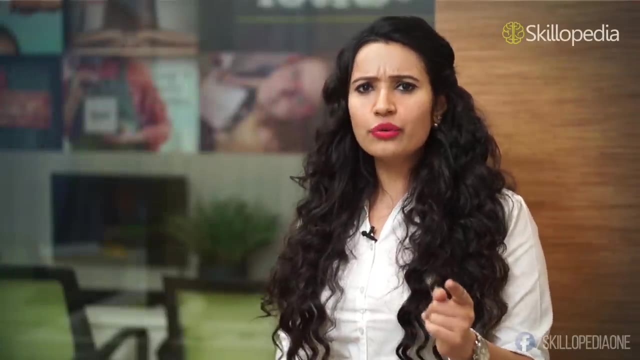 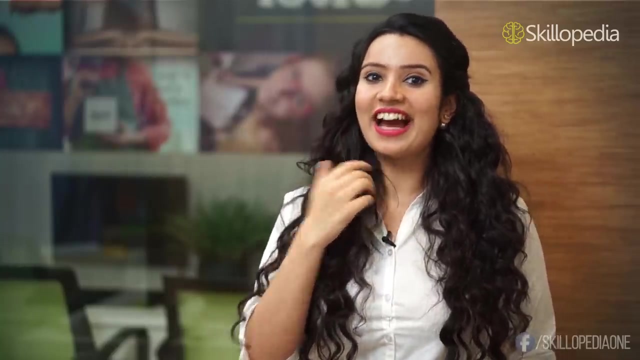 in for a great speech. The start of your speech is the most important part. Walk in your room smartly, lay your notes on the podium, look up, keep your chin high and greet them with a smile. Have a warm smile. Make them believe that you know what you're doing. It always gives. 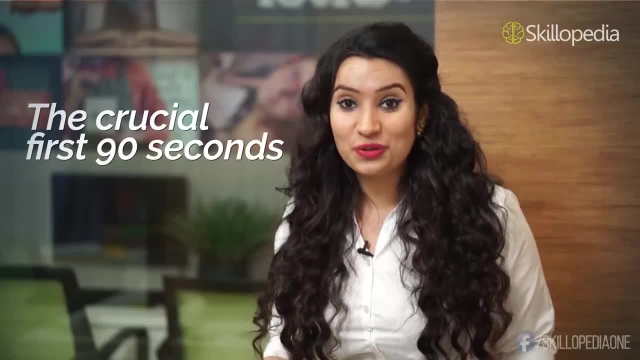 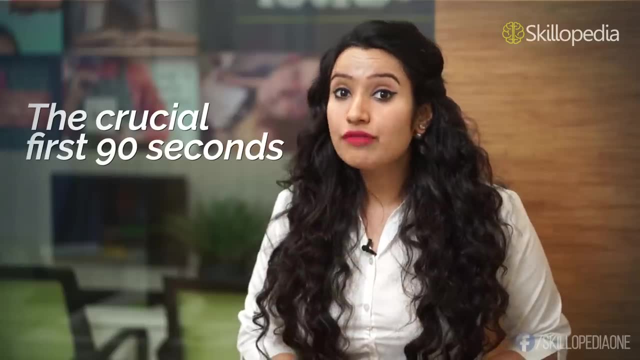 one a lot of comfort when the other one has everything under control. So if they think that you don't know what you are saying, that's going to be a problem. So be the one who has everything under control. The best way, I think, to capture the audience's attention is to 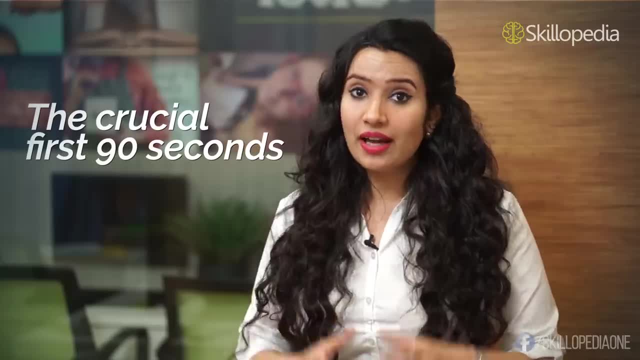 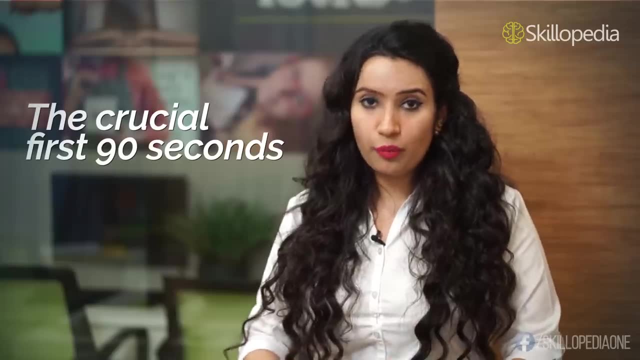 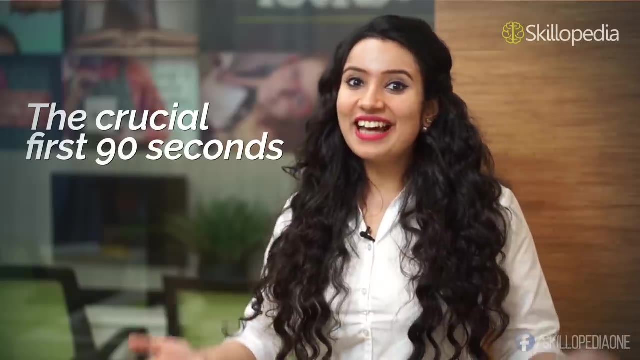 think about a clear and a strong phrase that people could relate to. When I was in high, was in school, I still remember the head boy would often come to the podium and raise his fist during the lunch break and say: defend your turf. What does that mean? That means: 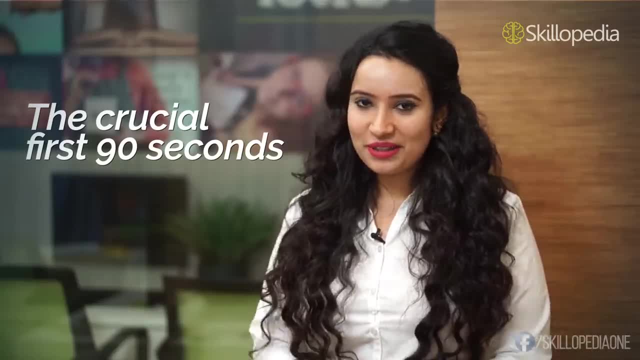 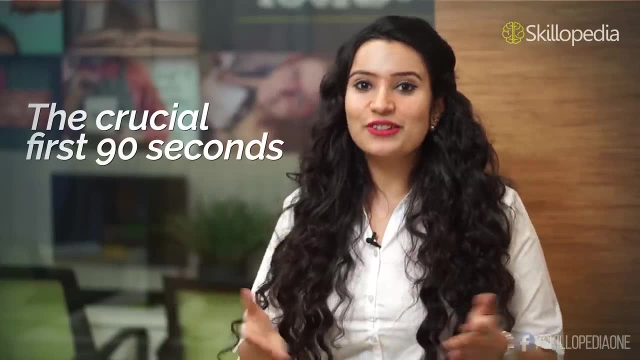 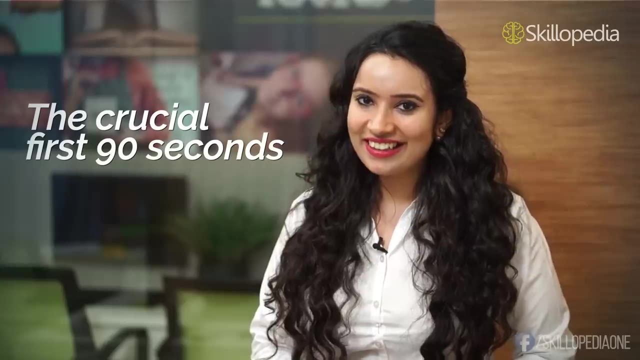 to take care of your belongings. Well, he used to say that because our bags used to be overloaded with food when we returned from our home after the winter break, So that used to make everyone laugh, and we all used to listen carefully after that to everything he said, Did you? 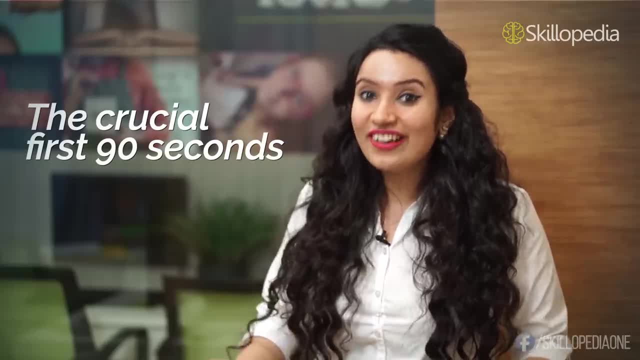 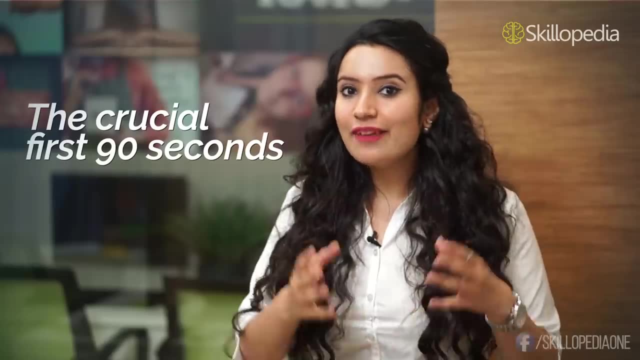 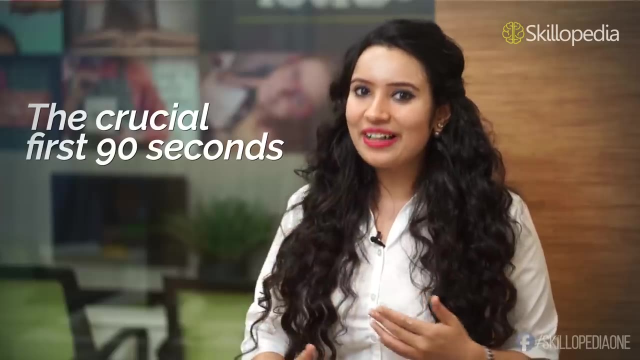 notice. all he did was he chose a strong, a funny and an interesting phrase to start his conversation, and this is what you should do If you want the audience to relate to you easily. it is always a great way to start the speech with a light-minded, nice and strong. 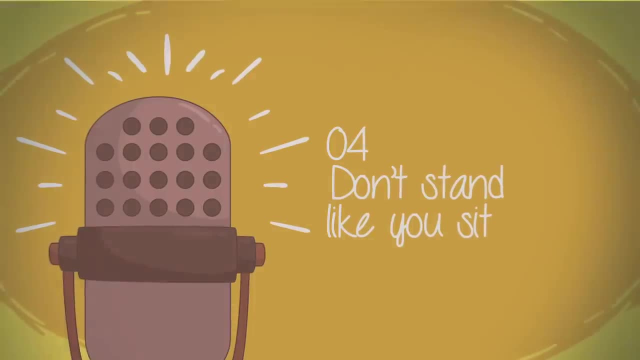 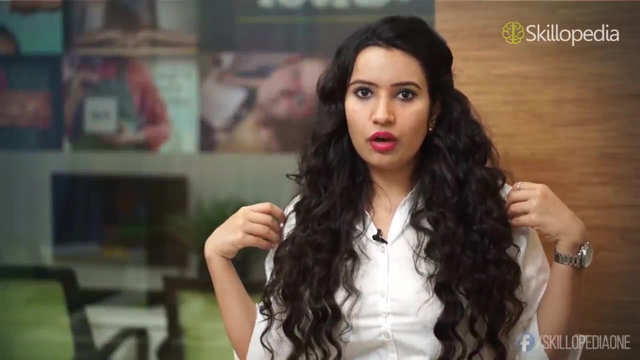 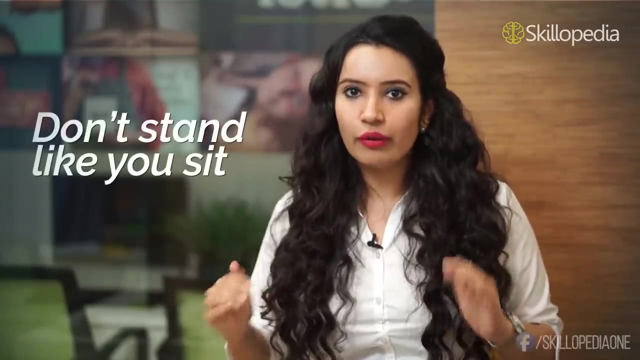 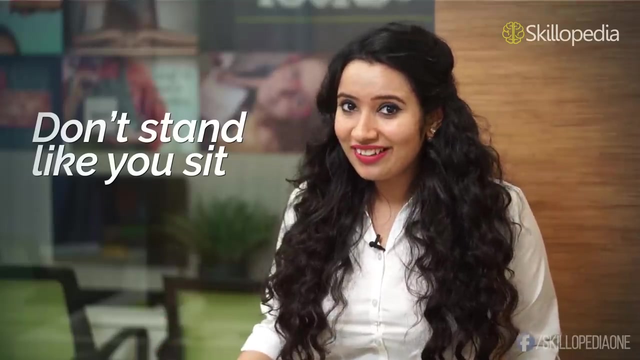 phrase that could capture their attention. Unfortunately, even though we are human beings, we stand almost like we sit, which is so horrible. Never has a person who has dragged himself on the stage slouching attracted anyone's attention. You know what I mean. Most of us don't realize that much of our confidence. 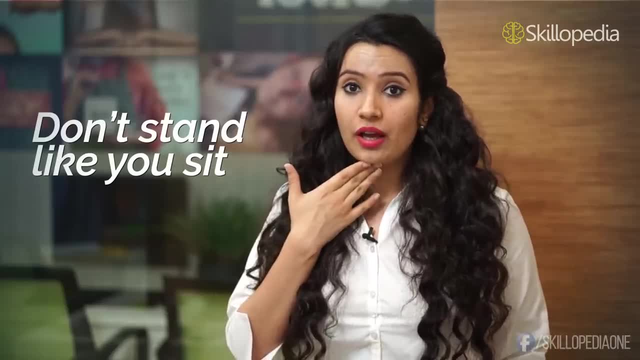 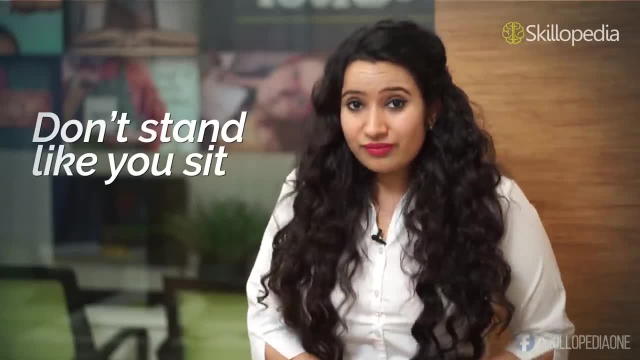 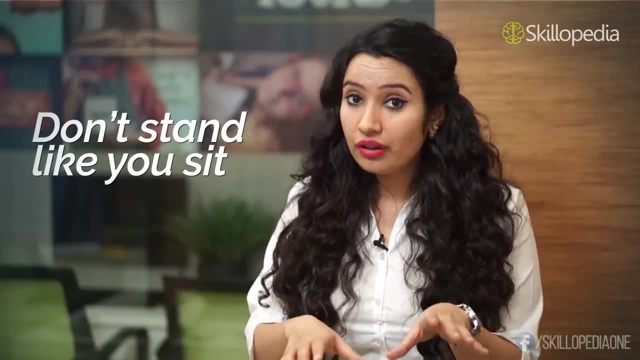 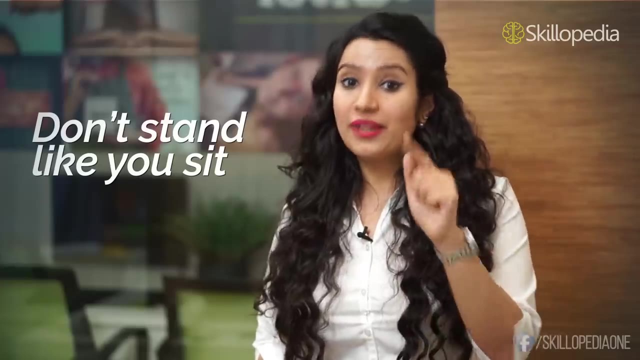 too confident, Too low often shows you are very nervous. What should you do? My suggestion is that you must observe yourself in the mirror by exploring different angles until you find the most appropriate one. Trust me, it will be a plus point when you have a good body posture, Curved back and slouching shoulders. 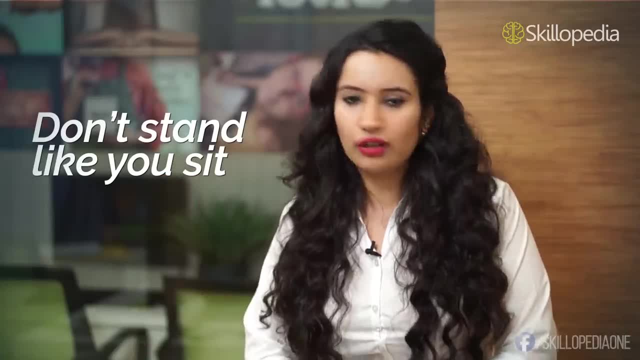 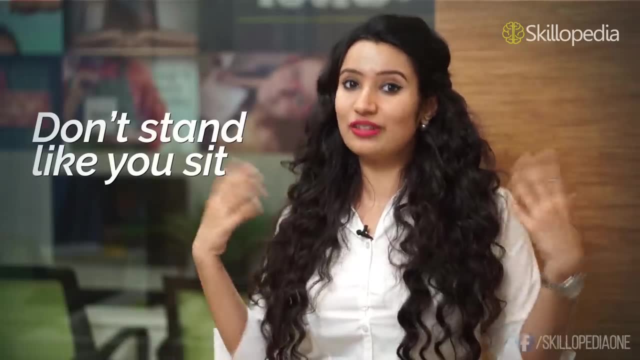 give the picture of a bookworm that has not left her seat for long. so that shows you've shows that you've been preparing for your speech for so long but you're not able to deliver it nicely because your body posture is not perfect. So if you can get taller without 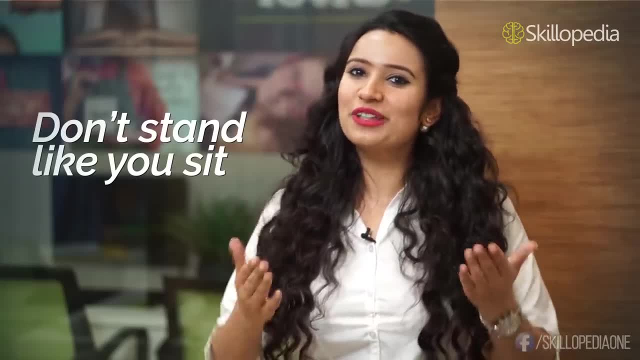 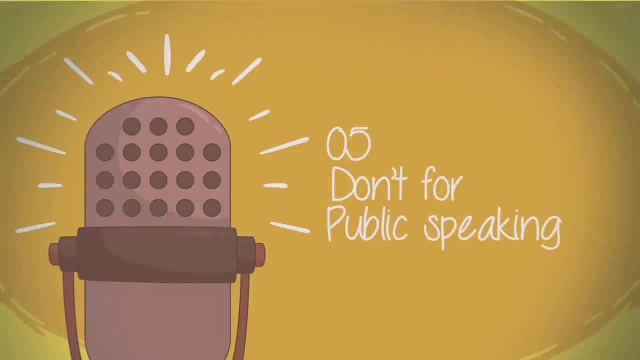 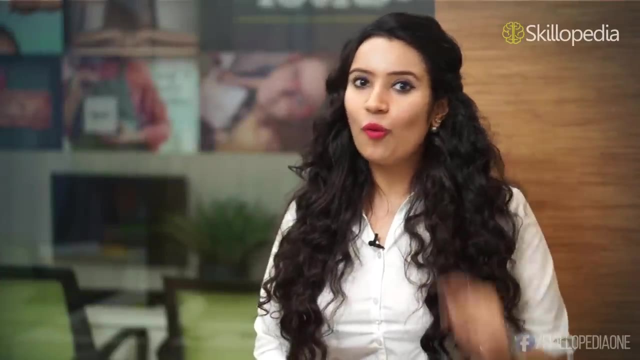 lifting your feet off the ground, then what you need to do is you need to make sure that your back is straight, and that's how you present yourself when you start your speech. Now let me tell you some things that you shouldn't do when you're speaking publicly. Kindly note. 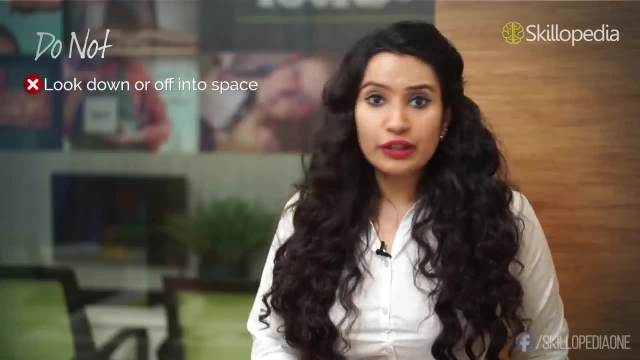 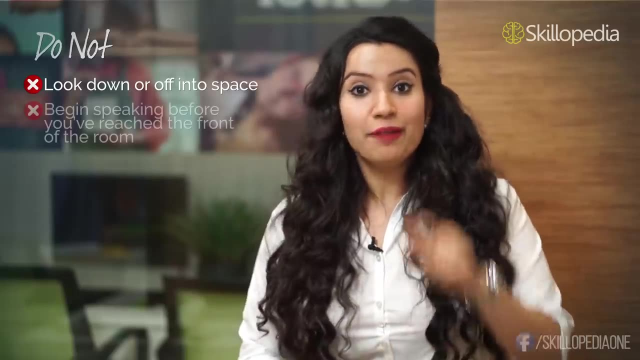 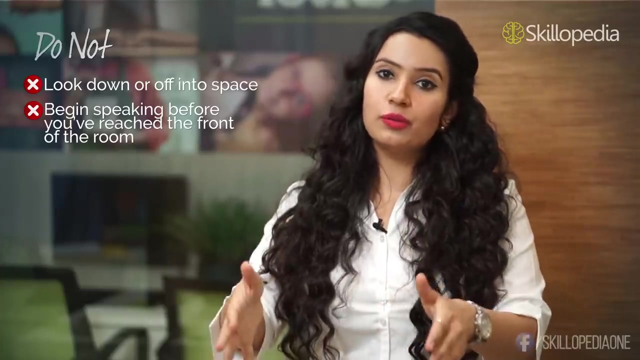 them down. You should not look down or off into space where there are no people. What I mean is you should make meaningful eye contact and please never start speaking before you have reached the front of the room. Start speaking when you're comfortable and when. 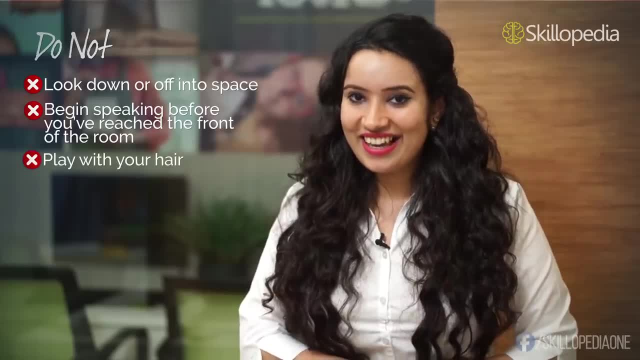 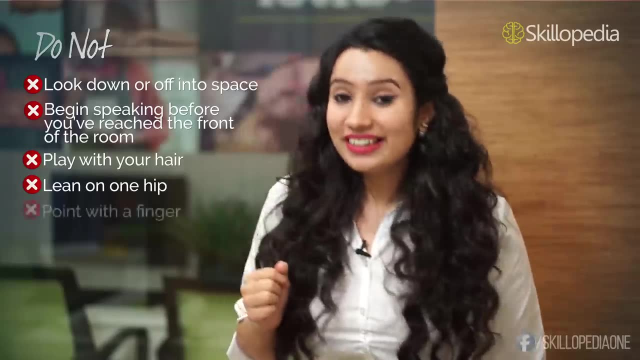 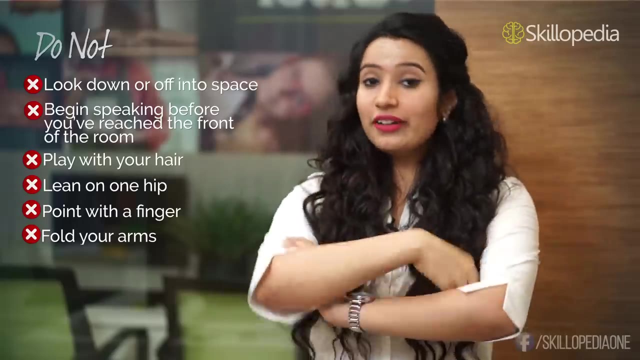 you're on the podium and you've got everything in place And, yes, please don't play with your hair, okay, Or lean on one side, and it's really not a good idea to point with the finger or to use an open palm like this, and I recommend that you don't.